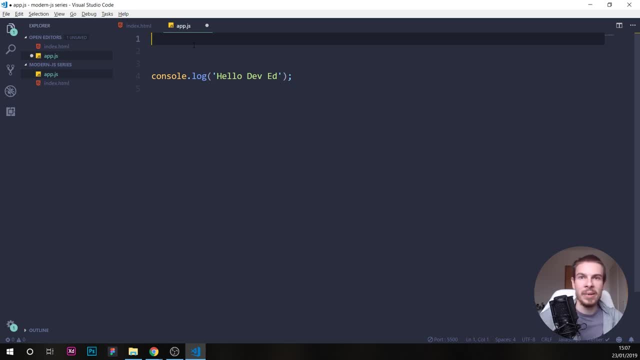 life bar would be a variable that's going to hold a number like 100 or however much life you need in it, So 100, and whenever you take a hit and you get damaged, you just subtract a number from it, So minus 10 or something like that. So then your variable is going to update, So your box is going 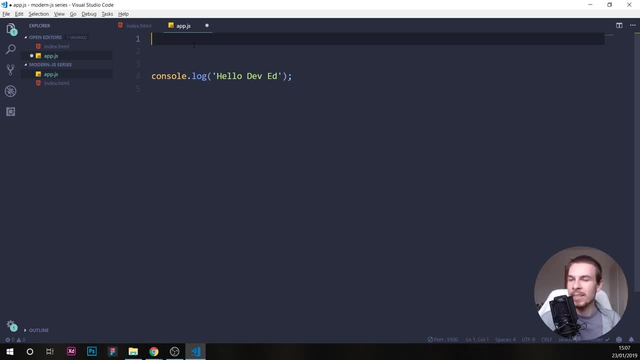 to update and then the new value is going to be 90. So 90 is going to be displayed, and that means that you need to practice because you took damage and you're not great at the game like me. All right, So how do we write a variable? Well, let's get ready. We're going to do it the old way and 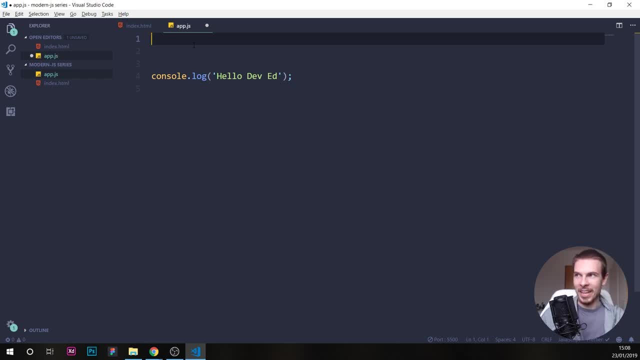 then we're going to do it the new way And I'm going to vaguely explain why we do this. So variable, how do we write one? Well, var like so, So variable var, okay, And then we need to. 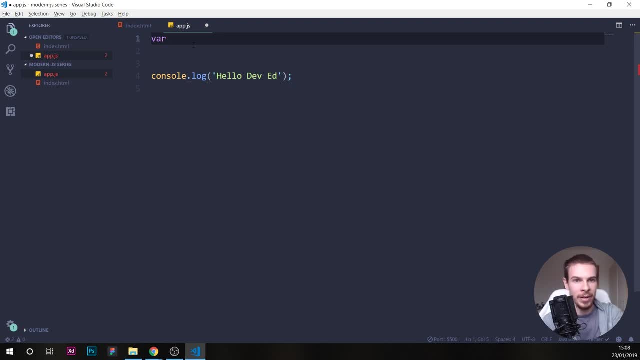 add a name to it. So what is our box name, our variable? Well, let's say life, because we use the game example And then we set it equal to, which basically means that we're assigning a value to it. okay, So what are we throwing in this box? This is what the equal means. And let's say we 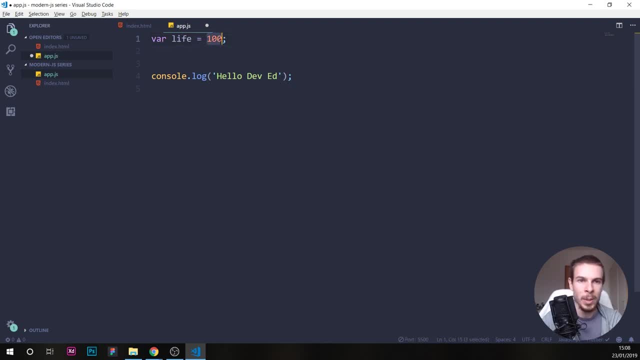 want 100.. So that's the number we want. We just write 100, simple, like so, And then we add this dot and this comma at the end. Now, why do we do that? Well, JavaScript doesn't really know what it does And it basically takes out all the empty space from here And when. 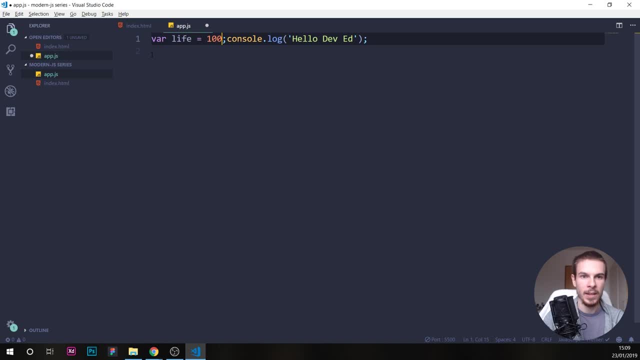 it runs. it's going to read everything in one line, like so: So if we don't have this dot and comma, it's going to read everything together like this, which is not going to make sense in the JavaScript world And it's going to throw a big fat error And I'm not sure what it's going. 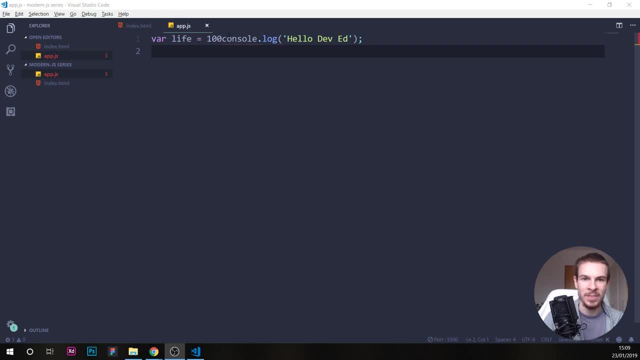 to throw, But let's see invalid unexpected token. All right, So it's just going to say: I don't know what the hell is going on here, Please fix, Please fix your bad code. So we add this, just so we know where our line ends. basically All. 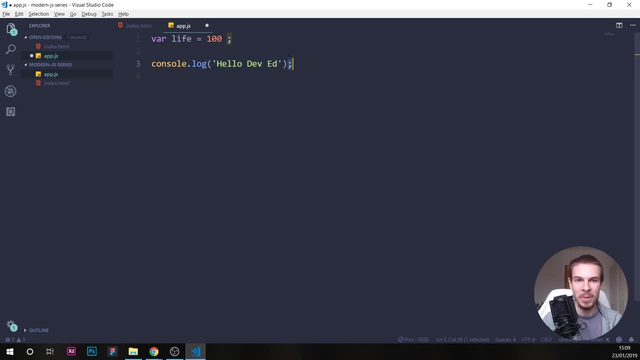 right, And that's what we did here as well. So we're going to use this every time we finish our line of code. Now, this is a number, Cool. What else do we have? Let's say we have some. let's say we have our name on the screen. So in our game, well, we cannot write like: 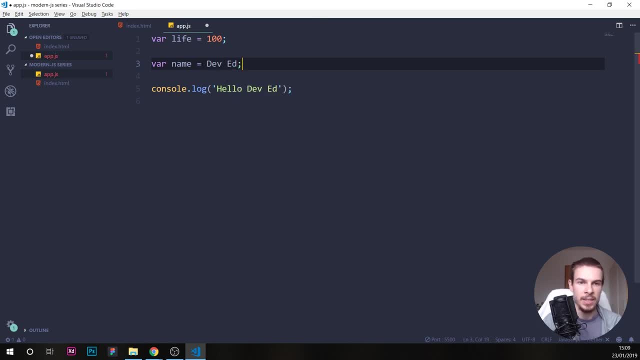 Deven Like so, because that means absolutely nothing in the JavaScript world. So, as you can see, here we added quotes which we can use here, And that is text. So this is valid, Because there are certain words that are reserved in JavaScript, So we cannot just 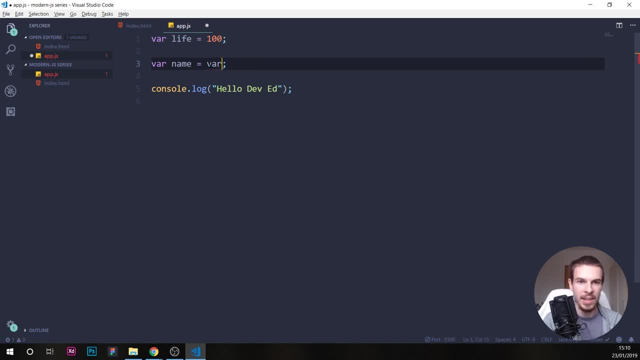 write var here or some things like that. That's not going to work because this is reserved. So to fix that, we can just add the quotes like: so, which is going to be string. This is going to be legit. It's going to work. It's not going to have any issues. we can add numbers. we can add anything. 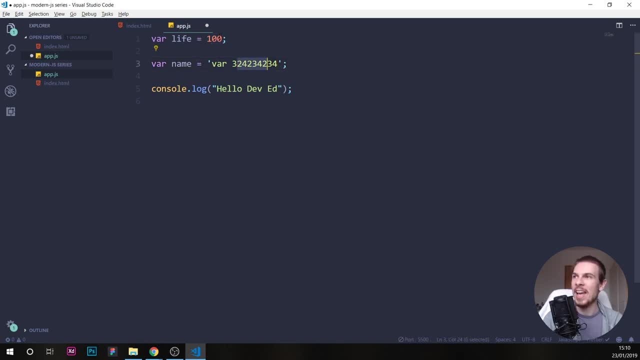 here. But the only difference between this and this is going to be that, hey, this is a number, with this number up here, we can do calculations. So we can subtract from this, we can add to this, we can divide it, we can multiply it, we can manipulate the number every way we want. But 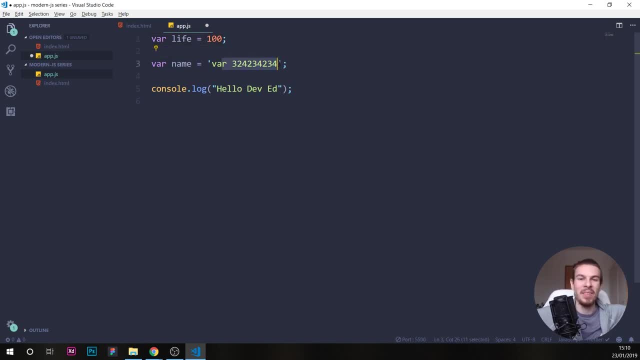 here. we cannot do that. we have different things. we can modify the text and uppercase it and add other different things to it, But we cannot play with numbers here, So we cannot subtract from this or add this. So this is just simple, simple text. So we're going to write dev at here as my name, Alright, so we have a live bar. 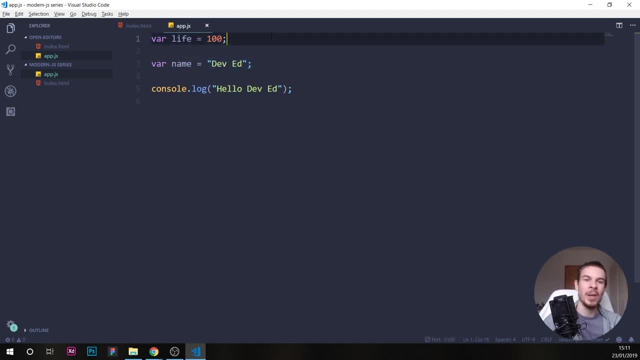 and we have a name. So what if we want to add, like notes to our JavaScript, like, let's say, we just want to let people know what this is? So to do that, we can just add a slash, slash, a double slash, and here we can write whatever we want. So this is not going to be read by 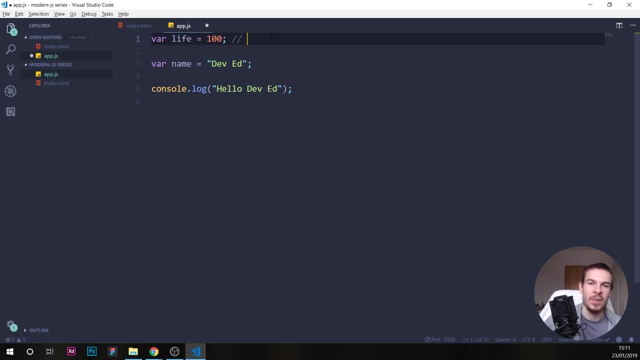 JavaScript. this is just going to be like adding notes to your code and letting people know, or yourself know, why and what did you write. So here we can say: this is my life bar, This is the name displayed in the game, And also this is a number data type, And this one is a string like so, So, 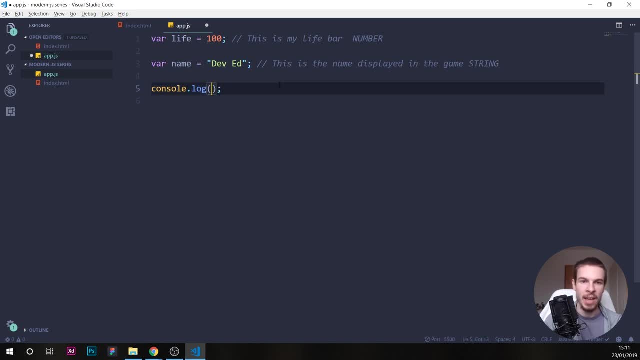 right now, what we can do is actually, we can delete everything we have in here And we can just add our variable, like so: So if we add life here and we hit save, we are going to have 100.. So rather than hard coding, so, rather than adding 100 here like so, we can just add life And it's. 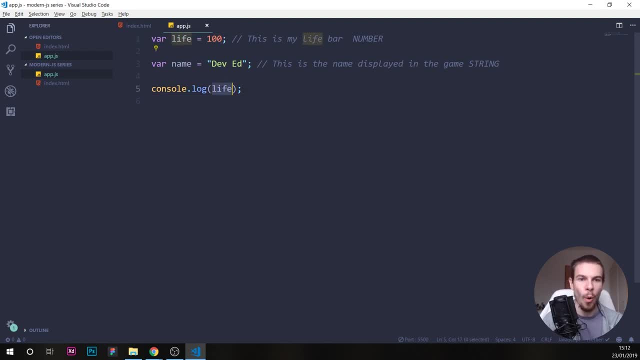 going to know that, hey, life is 100.. Or if we add name, not names name, we know that, hey, it's dev ed, Awesome. So what can we do here? Well, let's say we want to also modify this. So let's say we get hit, All right, our life is going to go down. So all you can do 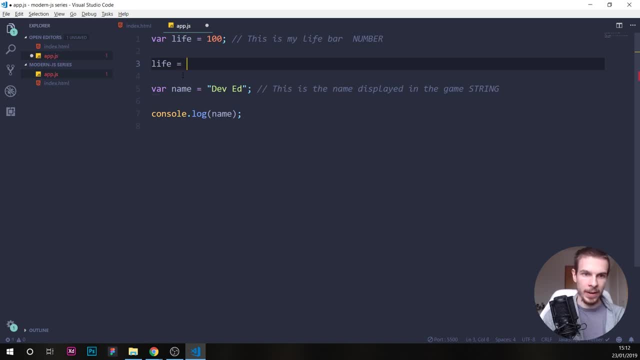 is say, life is equal to all right, so I'm, I'm getting the life variable and I'm changing its value again. So let's say we want our life to change to 50. So now when we console log the life, 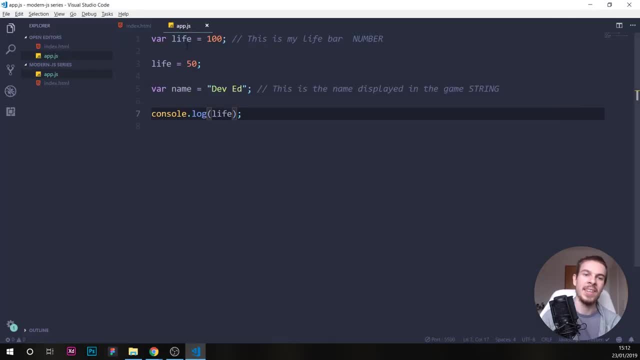 it's going to be 50. But what if we want to- let's say, we want to- subtract from the original number up here? there's something that you're probably going to do multiple times. Well, what we can do is because, let's say, you get damaged and you get damaged more, but you want it to start from this. 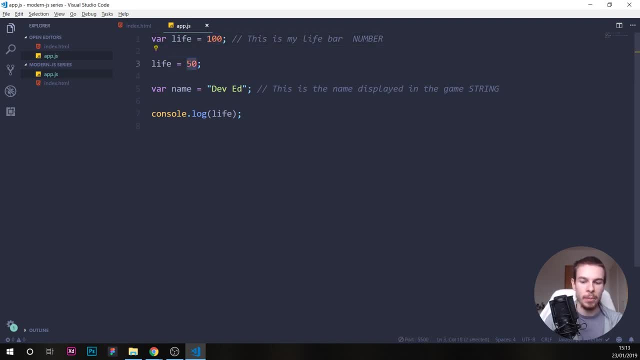 value and you want to get the value again. To do that, we can write life again here. So our life variable is going to equal to and again the value is 100. So this is going to be added dynamically in here, So you don't need to write 100 minus 10, like so, which is going to give us 90,, like so So. 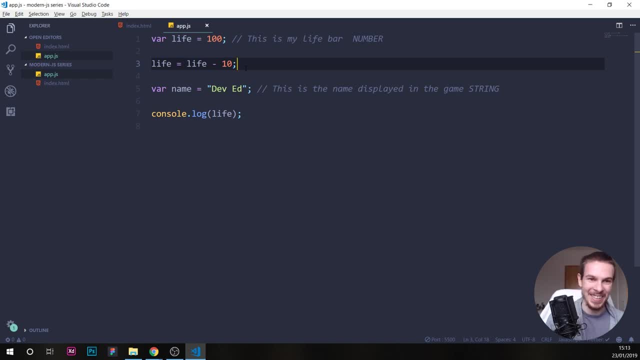 I know this looks kind of weird. It is what, it is what you're gonna do. But let's say we copy paste this, it's going to give us 80. Because what's what's happening here is we get the variable. 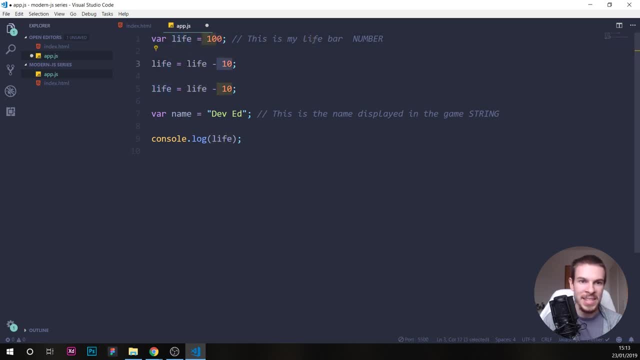 this is 100 minus 10, it's going to be 90. So, right here, our value is 90. So life is equal to 90.. And then we get: the life again is equal to well. now it's 90. So 90. 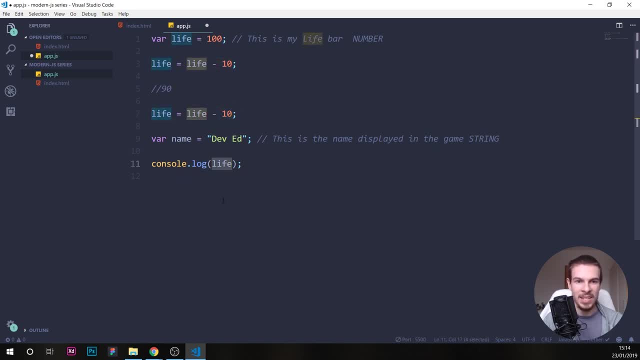 is going to be passed in here minus 10. Well, it's going to be 80. So that's why we get 80.. Here you can also do plus. here You can also do divide like so, And you can do multiplications like so. 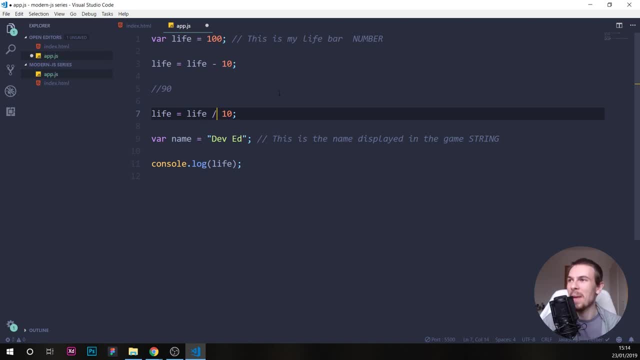 So you can use everything basic and math and more If you want to. we're not going to be going into complex algorithms, But these are probably going to be enough for most things. Cool, All right. So with text. I'm going to cover later what we can do. 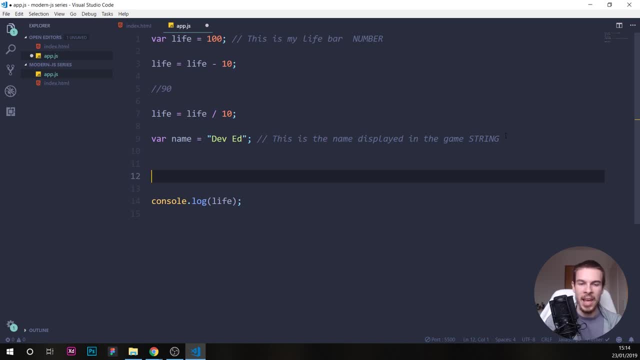 with this. But what, what, what else do we have here? Well, I'm going to cover one more, because these three are really probably going to be used. most is something called Boolean. So what's a Boolean? Sounds funny. Why is it useful? 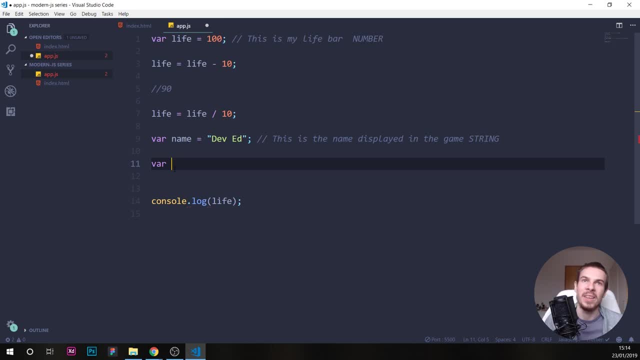 So let's say we want to do a shopping website and we have a checkout button- right. But we only want that checkout button to be available once we have a product in our baskets. right, Because if you don't have any products, why are you checking out? Well, it's just the empty box coming to your 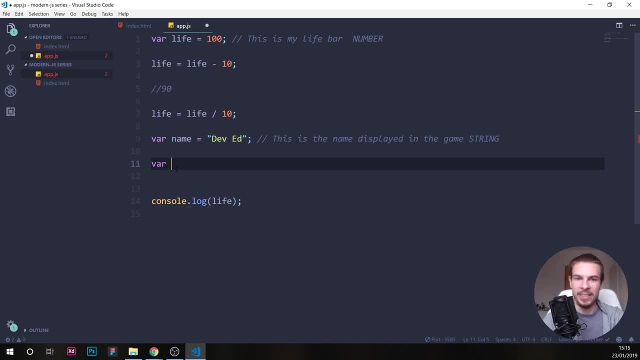 house. Hey, maybe I don't know, I'd still be excited for that. I like empty box, I just like getting packages in general. But what we can do is, let's say, we have a checkout, okay, And a Boolean is basically a value of true or false. So, false, like so. Again, this is a reserved. 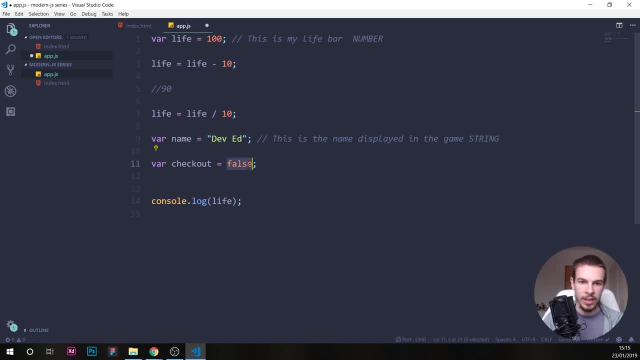 keyword. That's why we're not using quotes, either false or true. So in programming language thinking, you can imagine this like so: So let's say, if our checkout which is going to be true, then we can buy the product, All right, But if this has a value of, 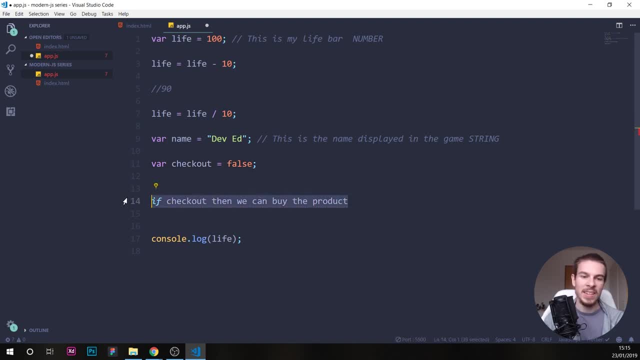 false, then this is not going to work. All right, So that's how you can imagine it. It's like a switch, like a turning the light on or light off, If the switch is on. if it's true, then you have. 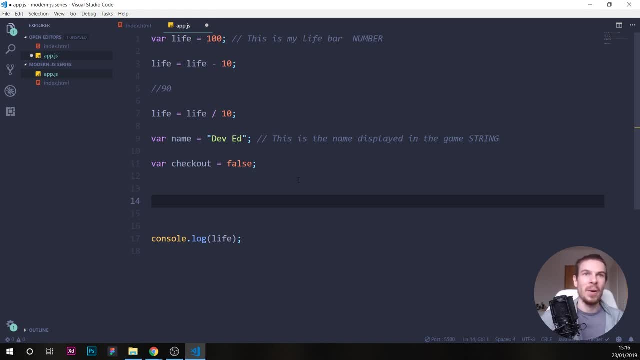 light. If it's false, then you have no light. So these kind of scenarios you can imagine like a switch type of thing. Hey, again with the check, like if you have a product, then it's your checkout button is true. If you have a product, then it's your checkout button is true. 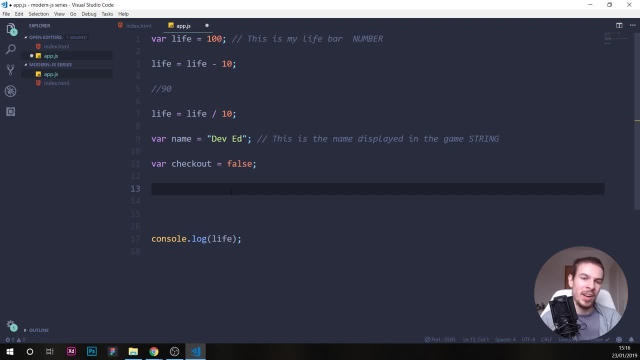 It's available, You can use it, You can click on it, You can order the product. So this is a Boolean And these are, and I'm going to cover three more, but I'm not going to go super in depth in them. 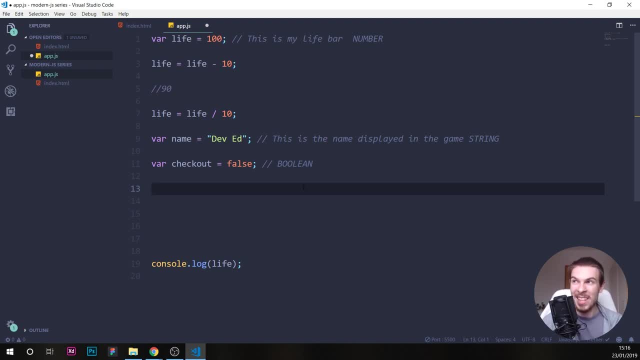 because, well, two of them are probably not that important, but we have one called undefined, which is basically, every time you declare a variable and you don't add a value to it, it's going to be undefined. So let's say var. 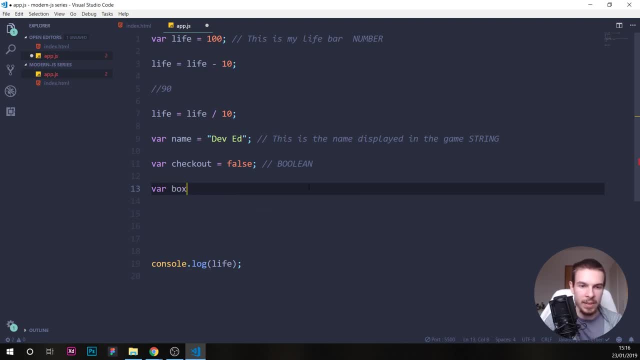 we're going to create, let's say, the box that we had, And I'm just going to declare it: like so, I'm not going to add equal and I'm not going to add a value to this. like so, All right, So what's? 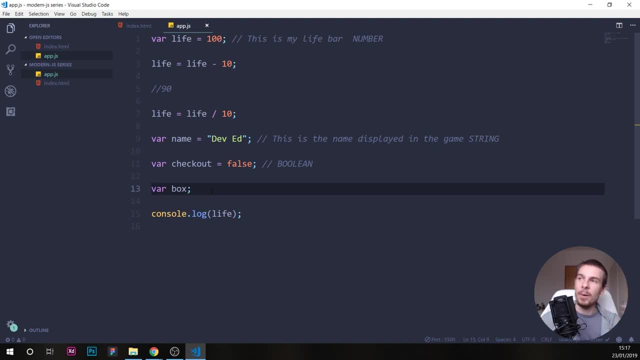 going to happen here. JavaScript is going to read this code and it's going to say: oh, okay, cool, We have a variable but it doesn't have a value, So I'm going to put it to undefined. So if we 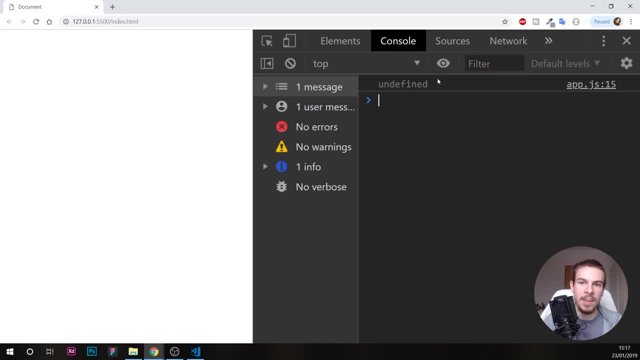 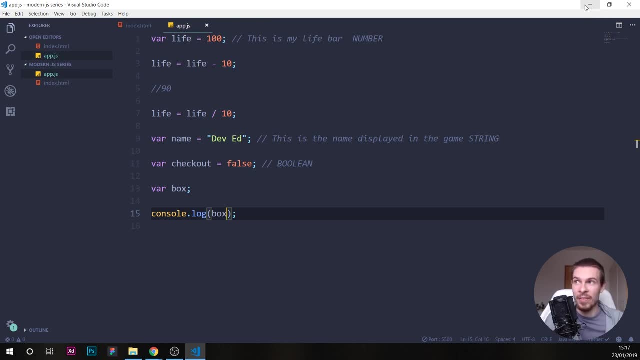 console log this box. it's going to say undefined. So that's basically what undefined is. It knows that there is a variable there, but it just doesn't have a value. There's also one called null, which we don't really use at all, But what this is going to say is that, hey, this variable. 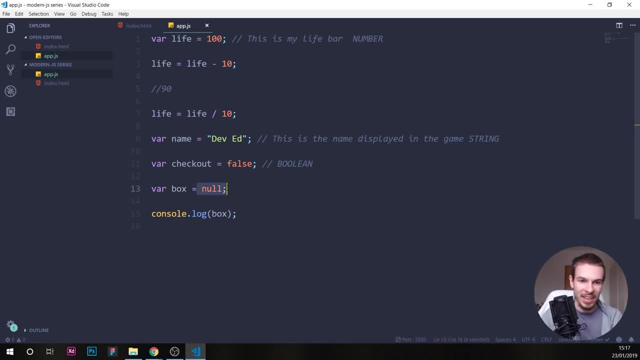 has no value. Okay, It has a value, but it's a non-value kind of thing. It's really weird. I know it can be a bit hard to understand, but rather than not having a value, it has a value of nothing. I know it feels like they were smoking. 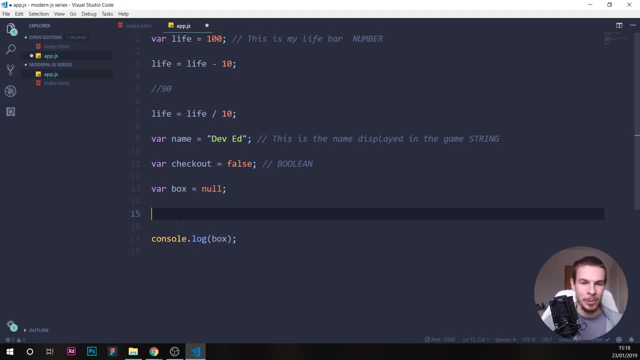 something when they create JavaScript, but it is what it is, All right. So we have null, and we have something called object as well- which I'm actually going to cover in later tutorial, So we're not going to be going too in depth with this- And also something called symbol- actually Symbol, like so. 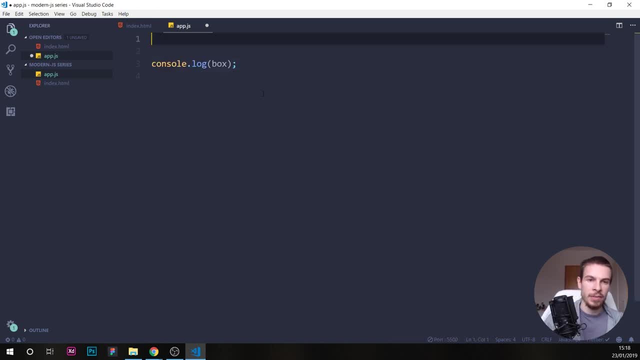 This is the old way, anyways, of creating variables. The new way is like: so I'm going to go super fast in this because there's just a few minor changes. So rather than having the var keyword, we have let and const. So the difference between these two is I just write const, like so is equal to 100. 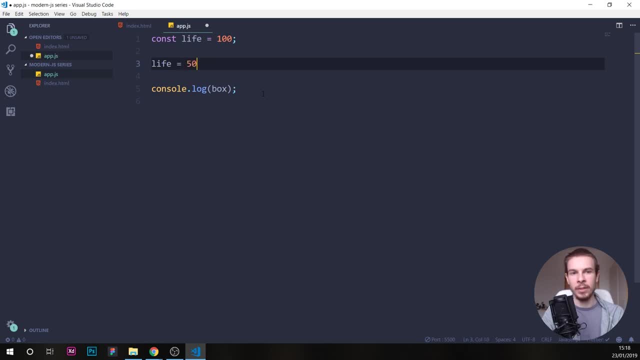 And the difference is, if we try to change this, so life is equal to 50, the const is not going to let us do that, So it's not going to. it's going to give us a lot of value, So we're going to have. 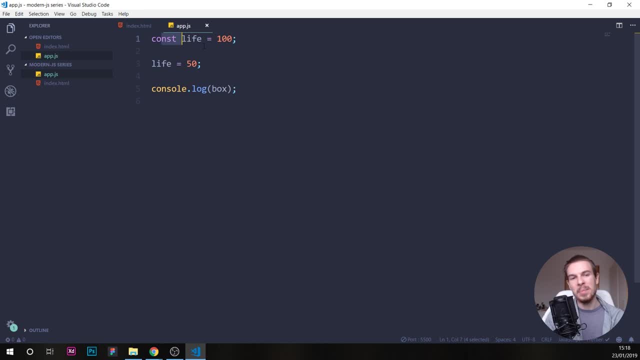 an error. It's going to say: hey, constant means that this value is going to be the same. So once you declare it, you cannot change it. So that's what const is. So we cannot modify the data in here, like so It's going to throw us an error. We cannot set life equal to 50.. And also one more: 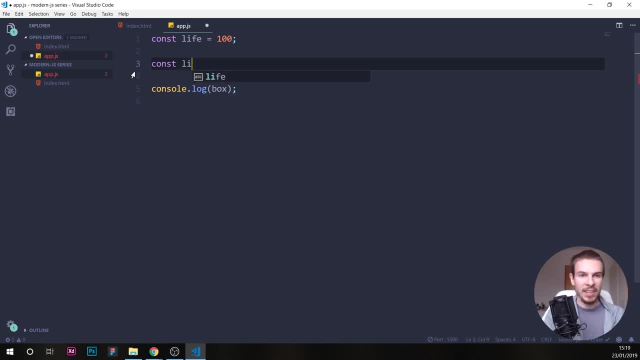 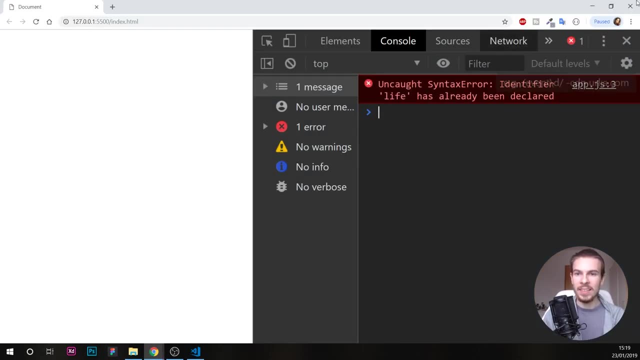 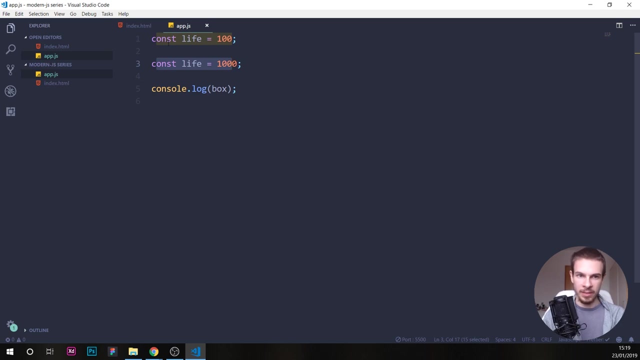 thing which applies to the let as well. we cannot redeclare the variable like: so It's going to say const already exists, So this variable already exists. You cannot just make a new one with the same name. We already have one. So it doesn't allow us to do that With var. you can do that. 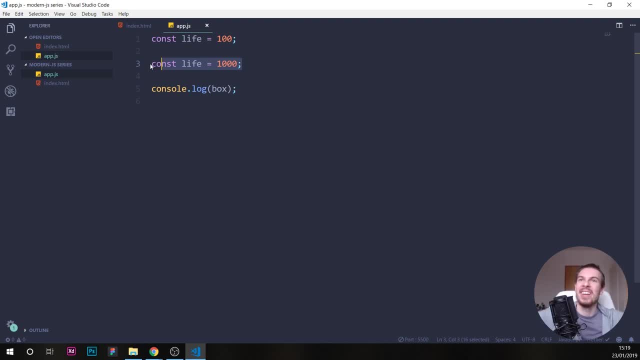 which is really bad because you might have, let's say you might have- a health bar variable And then later on in the code you redeclare another health bar variable which is going to change its value of the original And it's going to throw us a ton of different bugs And you cannot figure out what the hell is. 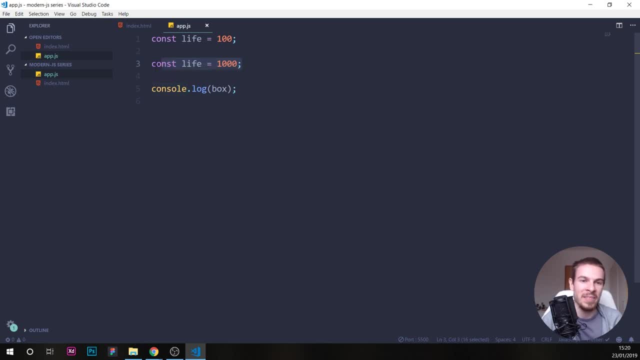 going on in your code, Because you redeclare the variable, which is going to basically change the original one, And you're going to have bad times. So this way, with the const, you're going to catch the error And everything's going to be nice and fancy. You know that. hey, maybe I need to use. 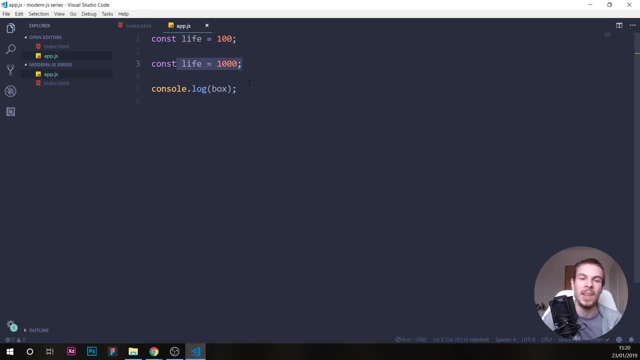 another name for this type of variable. Okay, cool. Now there's another thing that applies against const, And that's the variable that we're going to use, And that's the variable that we're going to use. And that's the variable that we're going to use, And that's the variable that we're.